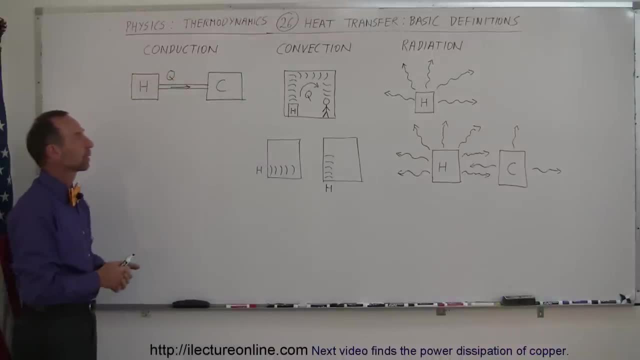 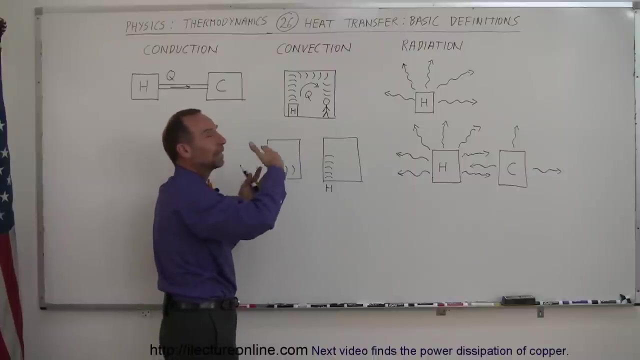 actually taking a road or path on that medium. Convection is a means by which which heat is transferred through the movement of the medium. For example, we have a hot object in a room. it heats the air up around it. the air will then move, expand and tends. 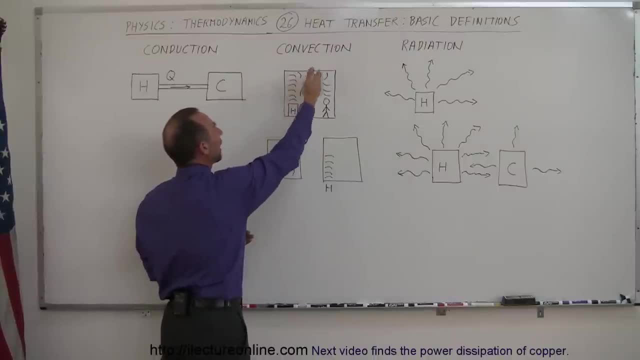 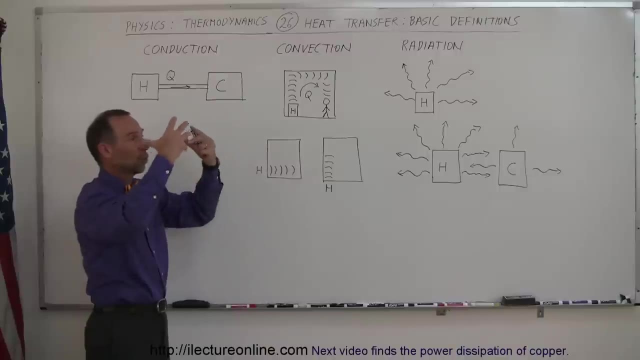 to move and the heat will then travel along with the hot air typically hit the ceiling, come around, then come down and heat a person on the other side of the room by having warm air move towards that person. So here the heat takes a ride on the medium. it's the. 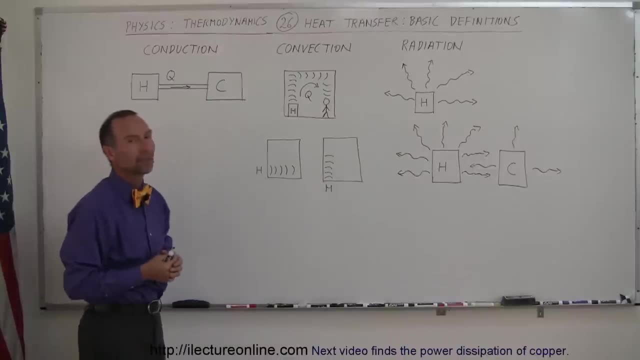 medium that moves and the heat just comes along for the ride. The third method doesn't need a medium at all, It doesn't need a path, it doesn't need something that it can go piggyback along, It just. radiation is just the means by which heat moves from one point in space. 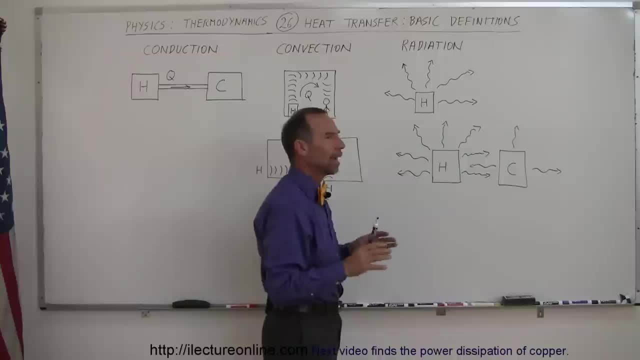 to another point in space, and it doesn't have to be anything in between. Now, there is space in between and space is something, but again we think of space as a vacuum that doesn't have any atoms within it, And so when heat radiates, 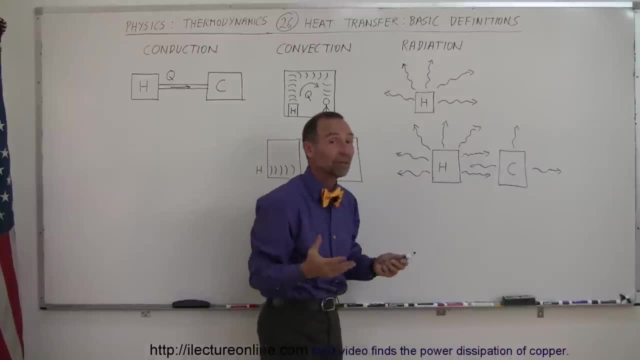 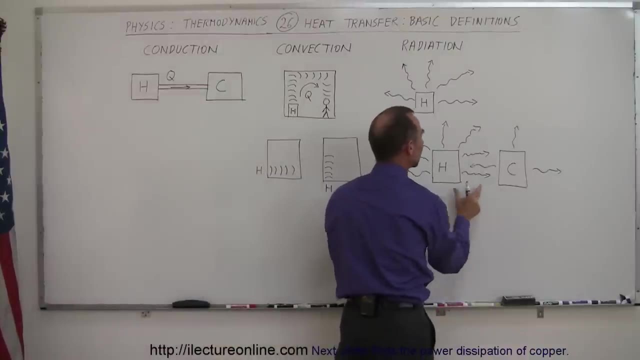 radiates out from a hot object. it goes in all directions, tends to go out at the speed of light. It's electromagnetic radiation, in essence, that moves out. And if you place two objects together, a hot object and a cold object, 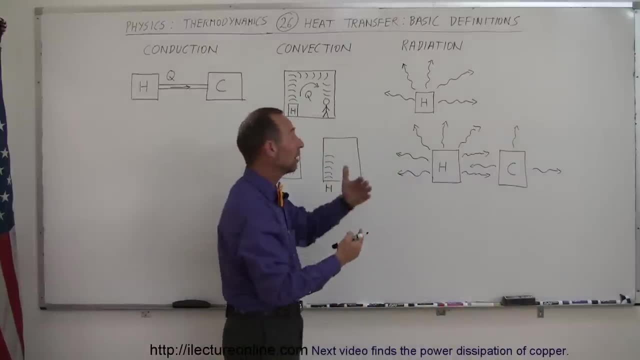 we will learn later that the hot object radiates way more heat and therefore cools down. A cold object will also radiate out heat and also cool down. However, if it's placed in the presence of hot objects, it will receive the radiation. 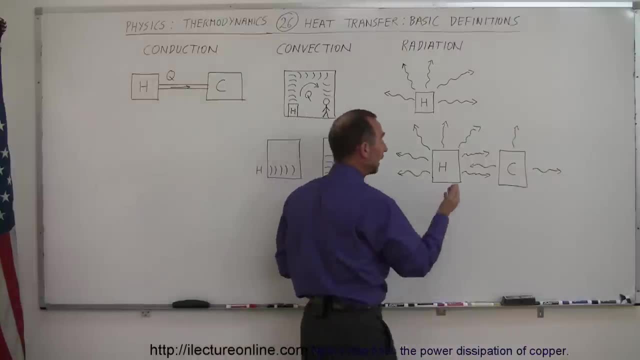 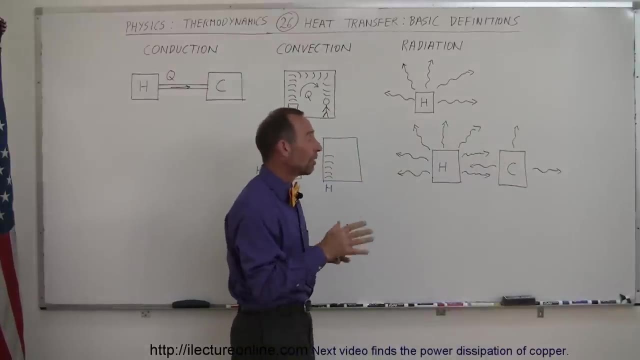 from the hot object, which tends to increase its temperature, And likewise the hot object will receive radiation from the cold object, which would tend to increase the temperature. However, since the hot object is radiating out more heat than it's receiving the net result. 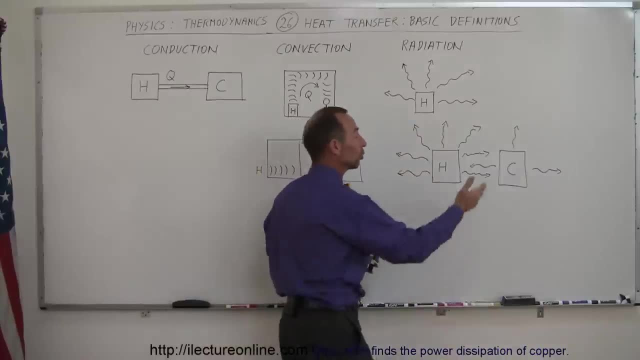 is that the temperature will go down for the hot object. Since the cold object is receiving more heat than it's radiating out, it will tend to rise in temperature And again, as you will see, in all three methods- conduction, convection or radiation- the temperature will go down.